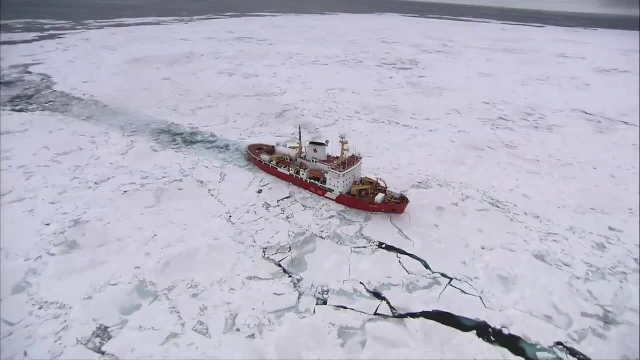 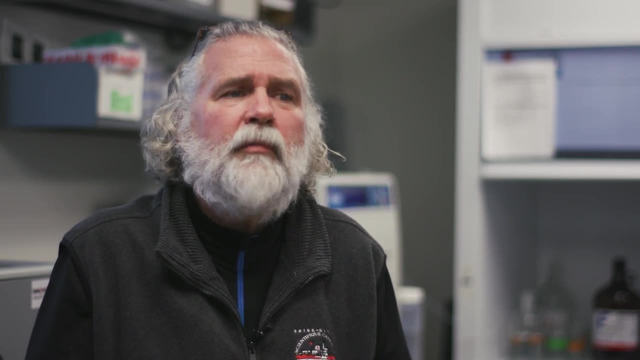 sea ice- Now multi-year sea ice- is that stuff that survives a summer and then goes to grow the next year and then survives the next summer, And that was typical of what we saw in the high Arctic basin. We're now down to 12% of the Arctic basin covered with that kind of 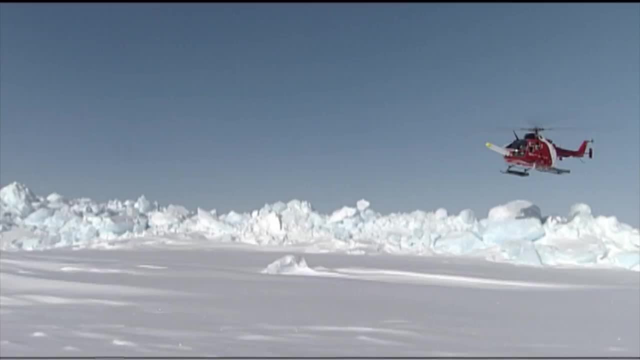 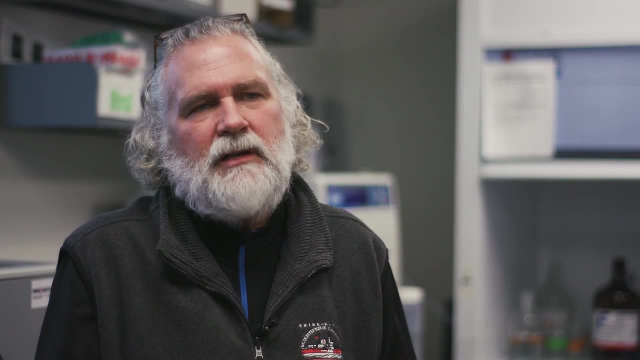 ice, And that has had huge implications throughout the system. Matter of fact, we don't see anything that isn't affected by that. So we went from something that had an average thickness of between 5 and 10 meters to something that has an average thickness between 1 and 2 meters. 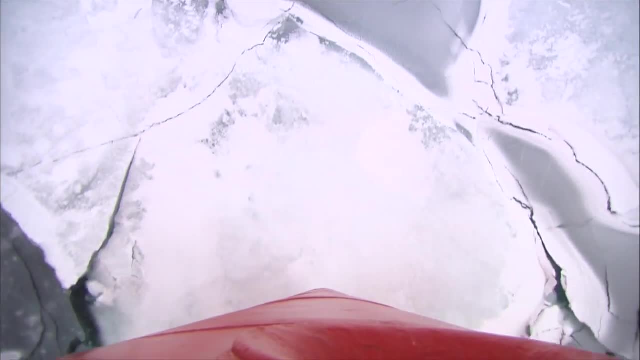 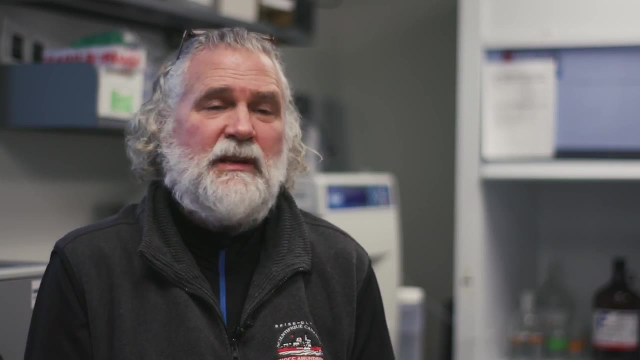 And so it's a very remarkable shift. Now that's affecting things in very complex ways, So we get involved with all of that kind of stuff, Like there's new forms of, or there's new species showing up in the Arctic, So the Atlantic, some of the species are starting to move into. 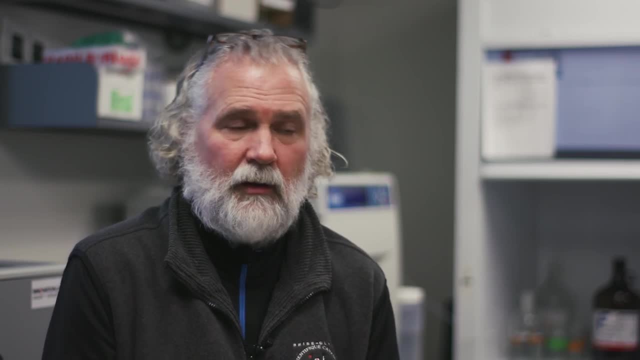 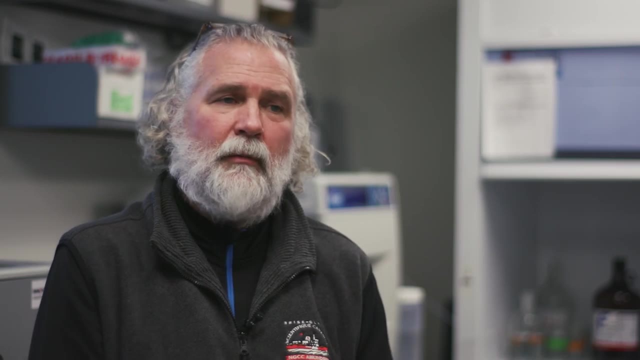 the Arctic And displacing the Arctic species. Same in the Pacific. It's happening on that side. Polar bears are a good one. People think about polar bears all the time as well. we're losing this sea ice, so that means polar bear habitat is disappearing, But in fact it's much more. 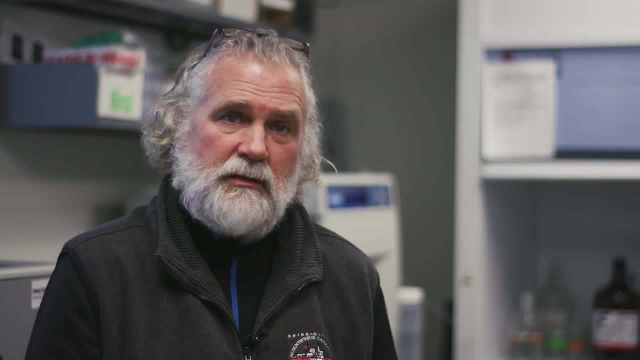 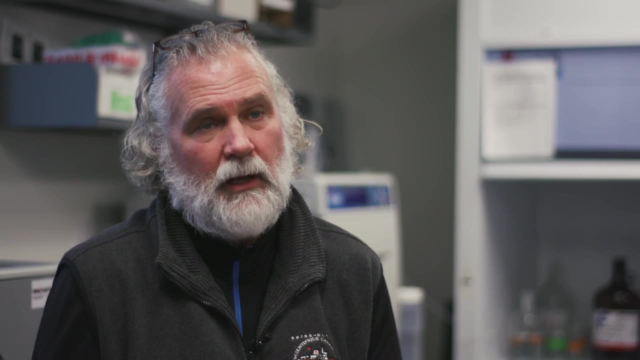 complicated than that, because the polar bears never used to use multi-year sea ice. They prefer first-year sea ice. So if it used to be dominated by multi-year sea ice, now it's dominated by first-year sea ice. It's actually improving habitat in some areas. The length: 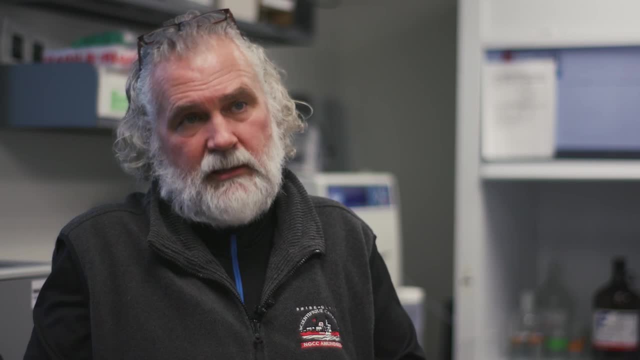 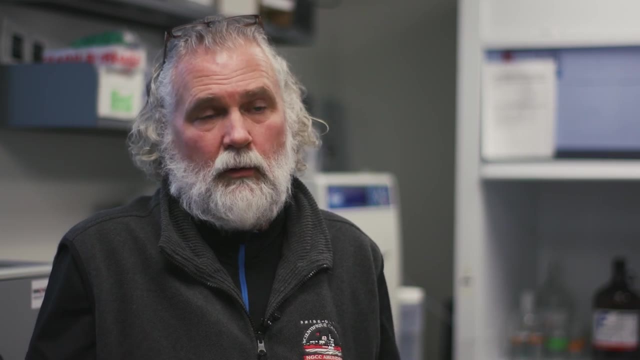 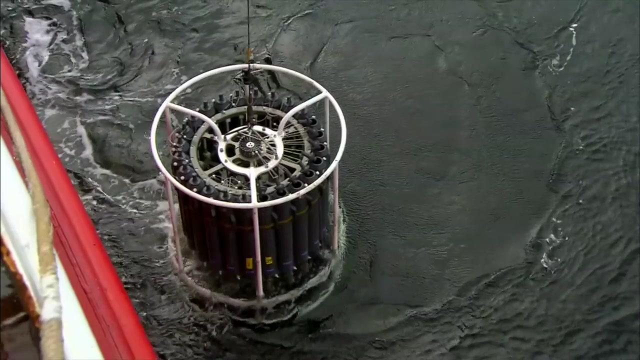 of open water season is what's really affecting them. So populations like Hudson Bay and the populations that are more southerly latitudes- they have to deal with more longer open water periods where they can't go out and forage for seals. I think on the technological front, we now have tools available to us that we never had. 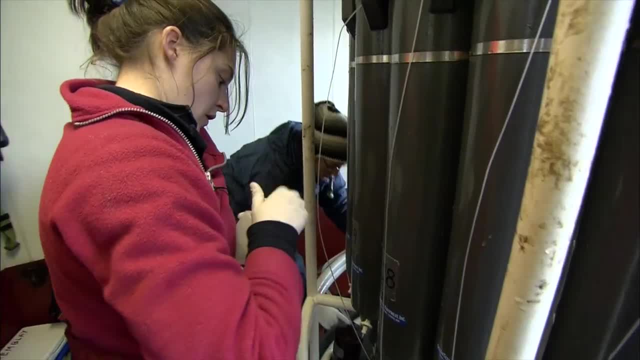 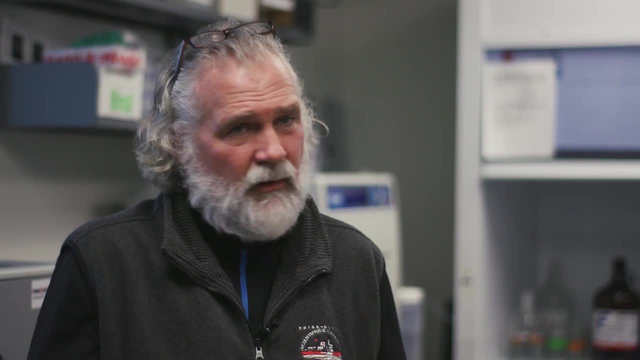 before. We can look at very complex things in the environment And in our lab. here, for instance, to give you an example, we start our studies at the nanometer scale, Like very, very minute, tiny kinds of scales, The kinds of instruments you see in this lab, are able. 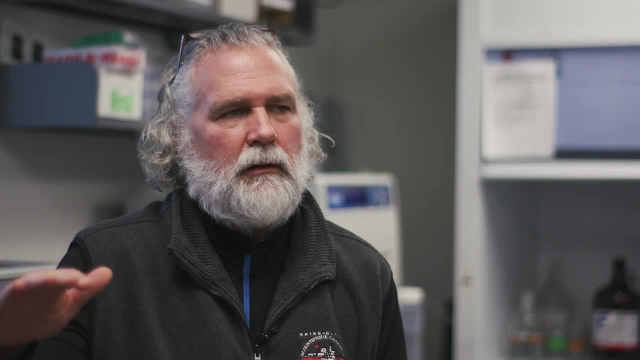 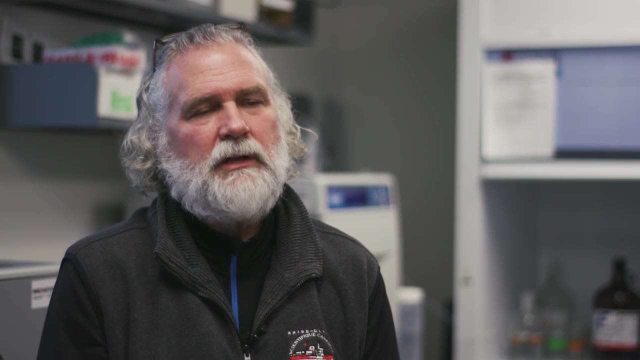 to do that kind of research And we go all the way up to looking at the Arctic from space And we understand all those different interconnections because of the tools we have. These tools allow us to do that kind of thing And then major investments like CMO. You know that's. 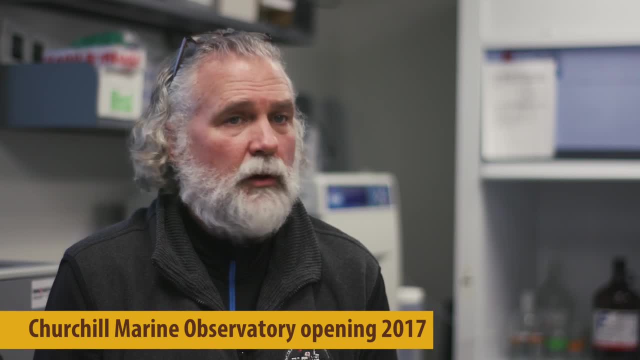 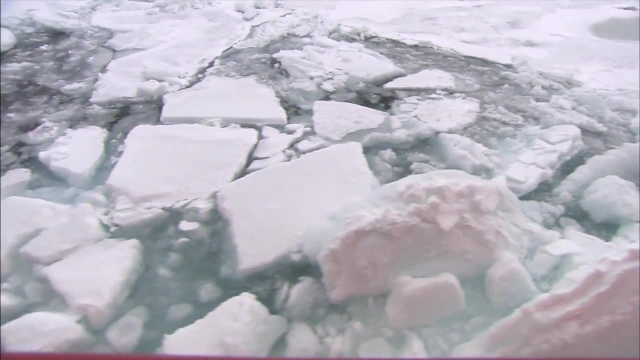 a major investment. It's a $32 million research infrastructure which is globally unique, which will really catapult our research. The same could be said for the Amundsen. Before the Amundsen came along, we were always restricted to just ships of opportunity in Canada, And